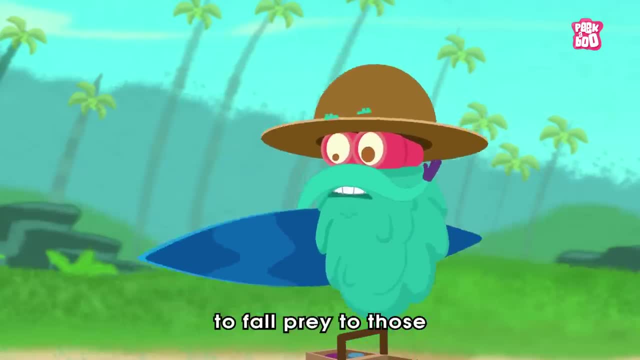 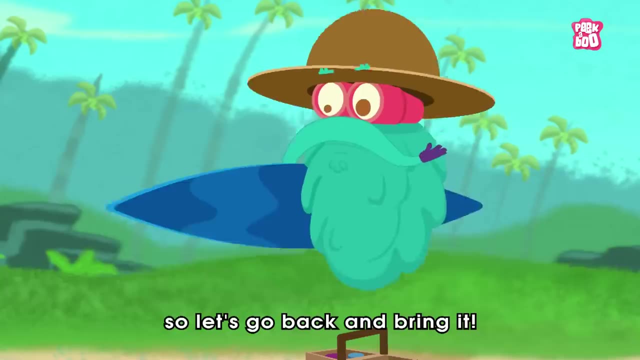 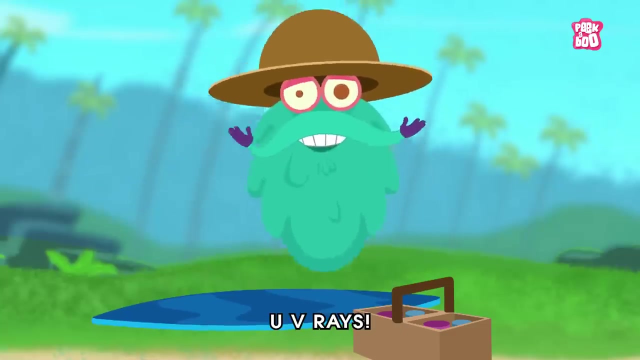 And I don't want both of us to fall prey to those hooligans. Let's get rid of the harmful UV rays from the sun and get painted with a tan. So let's go back and bring it. UV rays. Yes, little Kitty, UV rays. 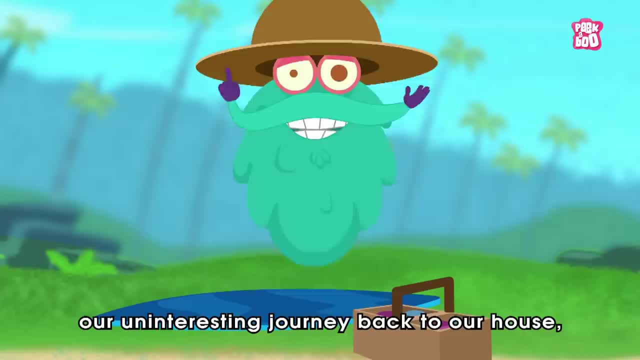 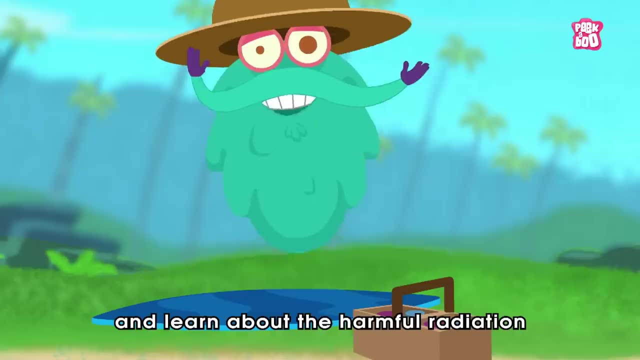 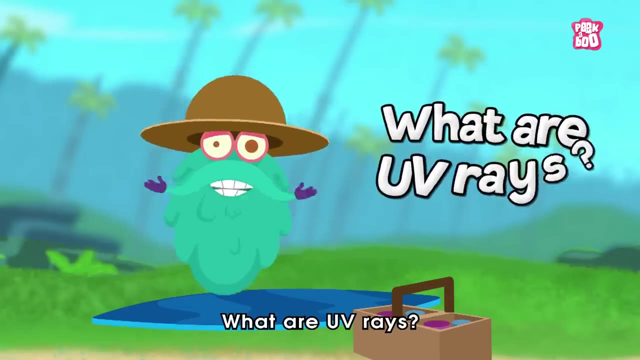 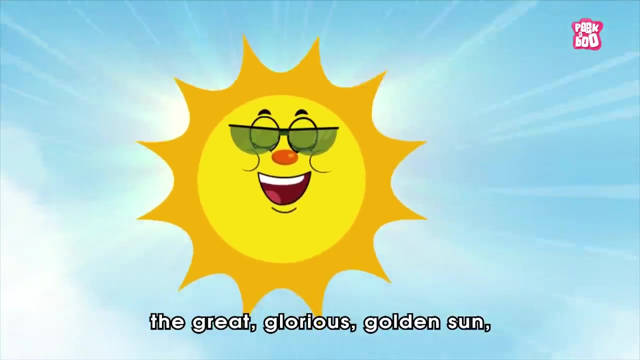 Hey friends, as we carry our uninteresting journey back to our house, let us fill it with some interesting discussion and learn about the harmful radiation coming from the mighty sun. and answer a burning question: What are UV rays? Zoom in The sun, the great, glorious, golden sun, the one that provides energy to living beings. 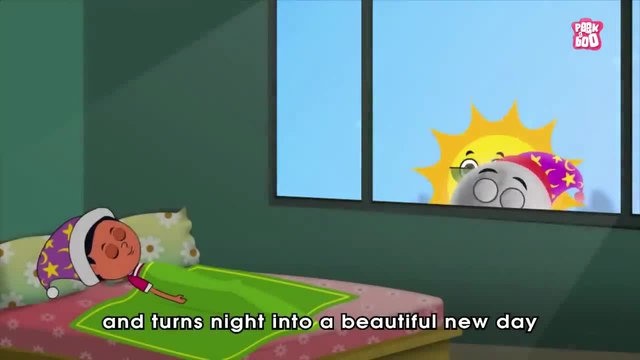 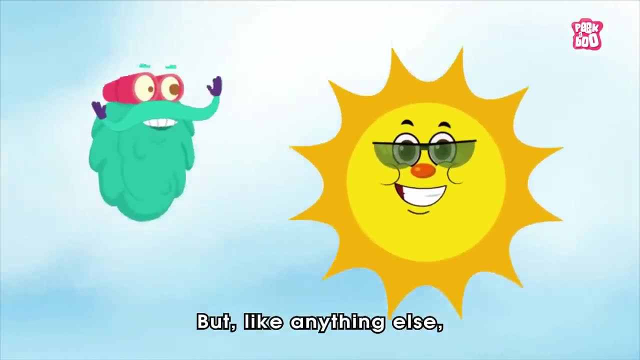 warms us and turns night into a beautiful new day filled with hope and enthusiasm. But like anything else, our sun isn't perfect as well and has a dark side to it. But like anything else, our sun isn't perfect as well and has a dark side to it. 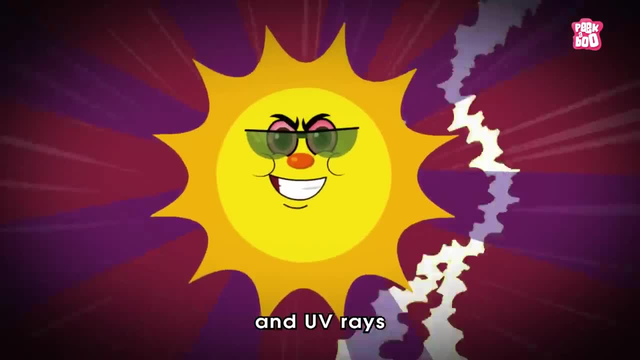 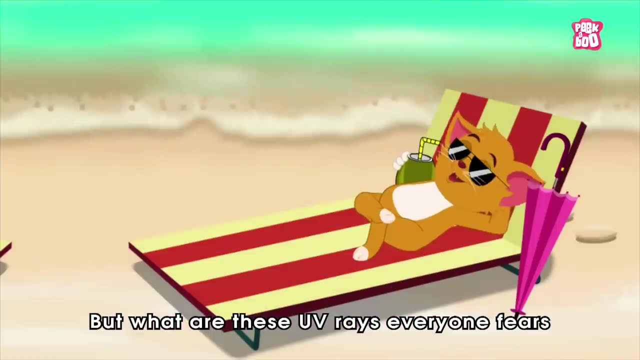 But like anything else, our sun isn't perfect as well and has a dark side to it. Yes, my dear friends, and UV rays are one such disadvantage our sun possesses. But what are these UV rays? everyone fears more than an asteroid hitting the earth's surface. 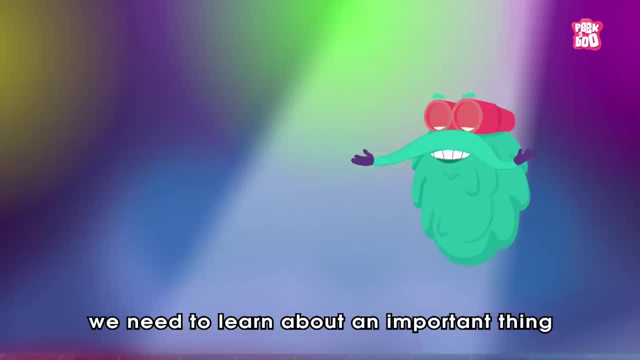 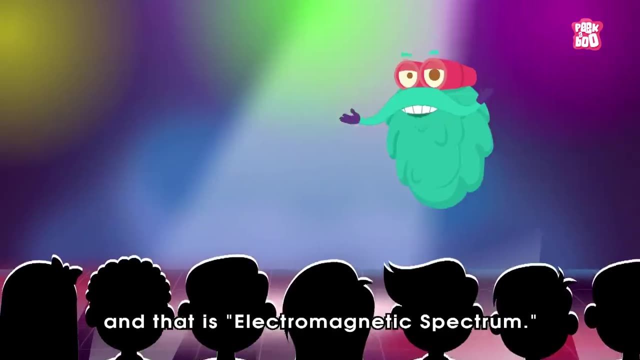 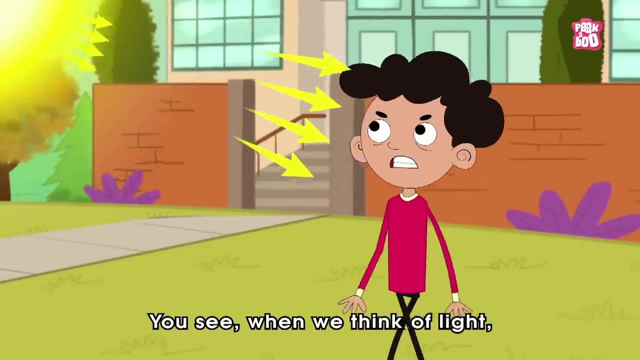 Before we answer that question, we need to learn about an important thing with a fancy name that sounds like the next sci-fi movie, And that is Electromagnetic Spectrum. You see, when we think of light, you probably think of what your eyes can see. 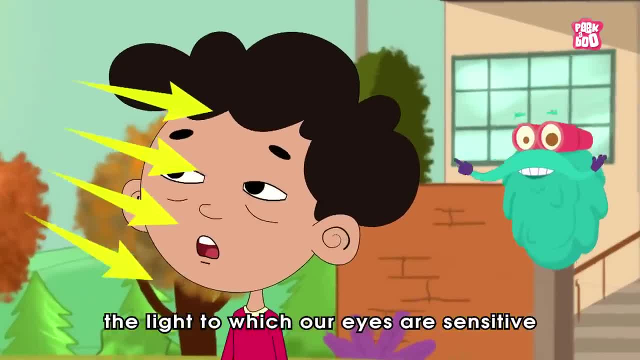 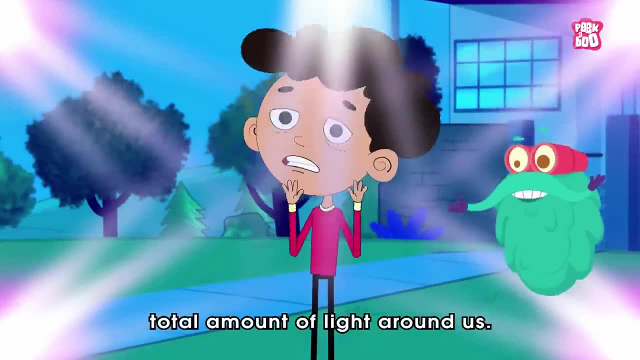 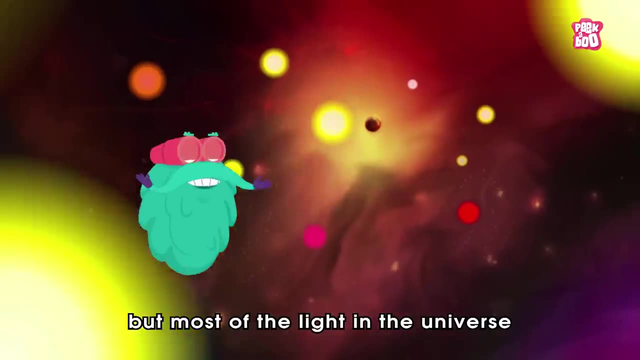 But the light to which our eyes are sensitive is just the beginning. It is a fragment of the total amount of light around us. Yes, right from radio waves, gamma rays, And you won't believe, but most of the light in the universe is invisible to us. 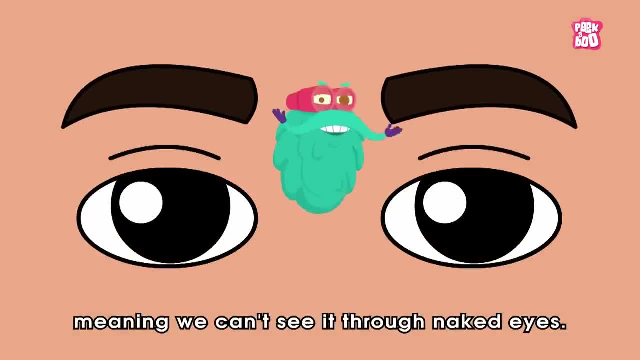 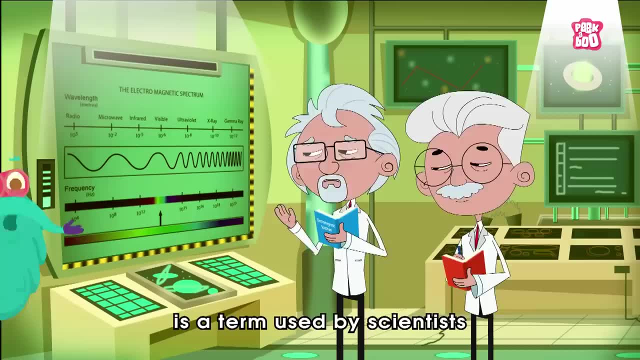 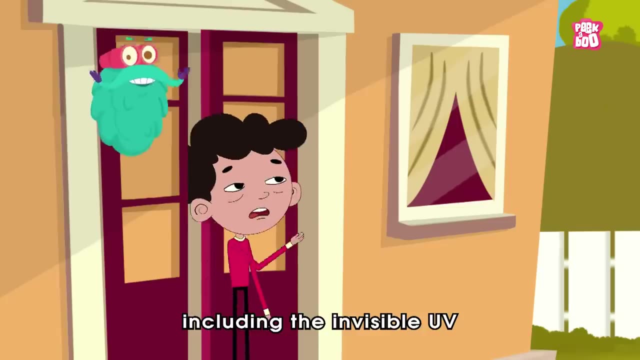 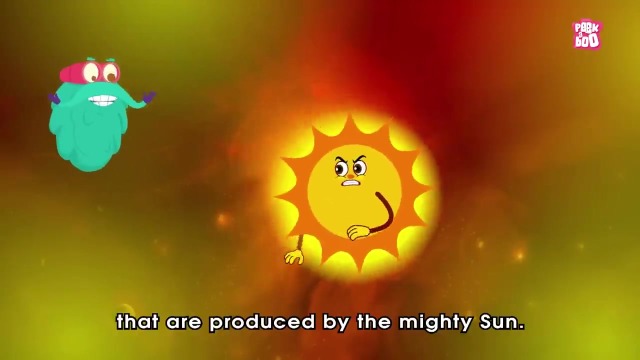 Meaning we can't see it through naked eyes. How ironic, isn't it? So? Electromagnetic Spectrum is a term used by scientists to describe the entire range of light that exists, including the invisible UV or ultraviolet rays That are produced by the mighty sun. 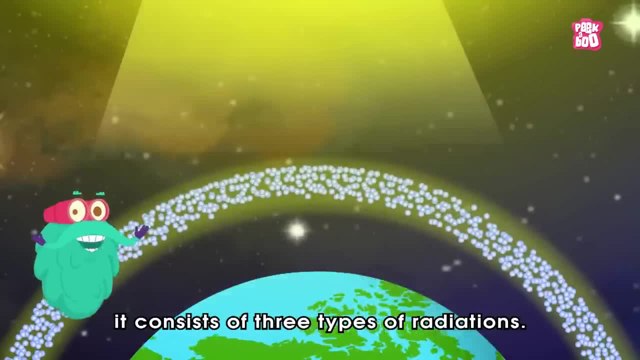 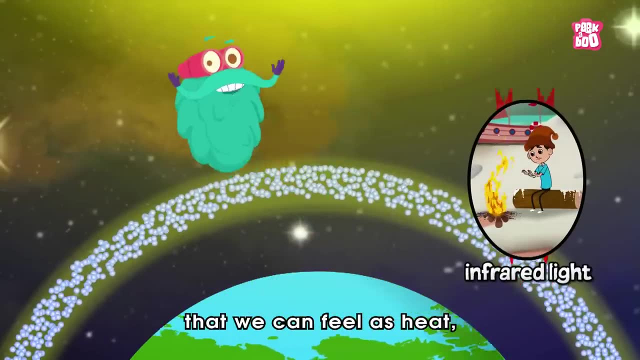 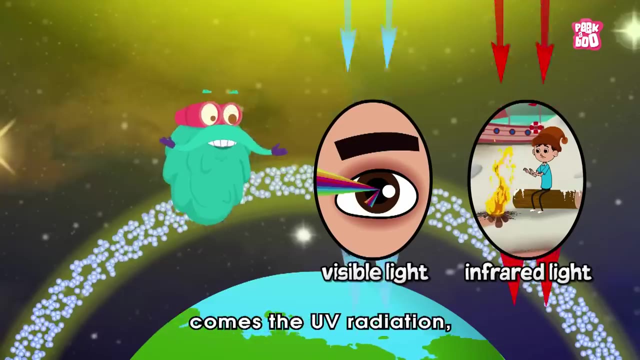 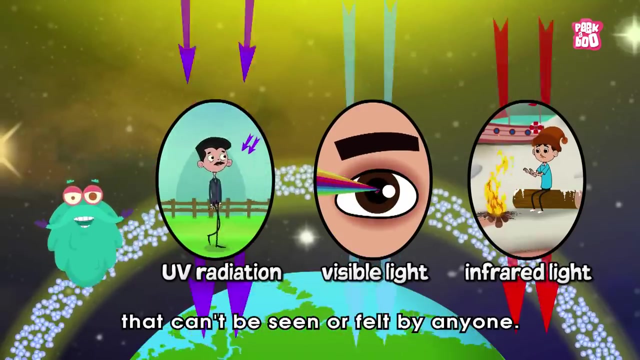 When the sunlight reaches the earth's surface, it consists of three types of radiations: The infrared light that we can feel as heat. The visible light that allows us to see the surrounding things. And last comes the UV radiation, The ever powerful one, that can't be seen or felt by anyone. 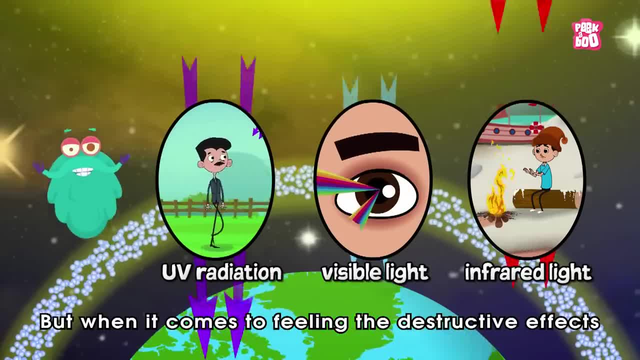 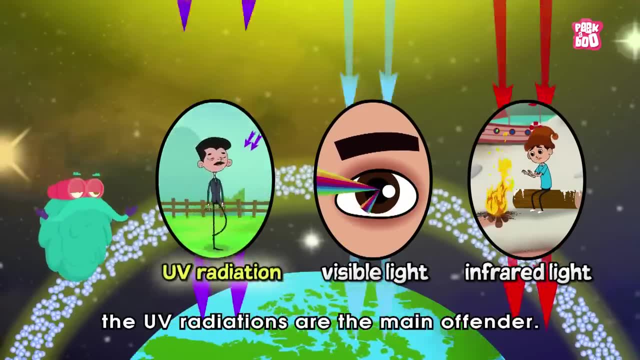 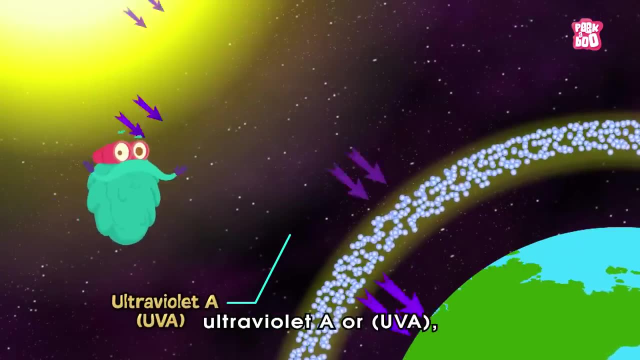 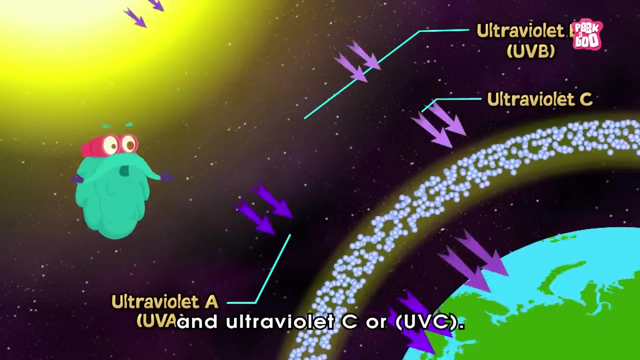 But when it comes to feeling the destructive effects of the sun's rage, the UV radiations are the main offender. These rays come in three forms: Ultraviolet A or UVA, Ultraviolet B or UVB, And Ultraviolet C or UVC. 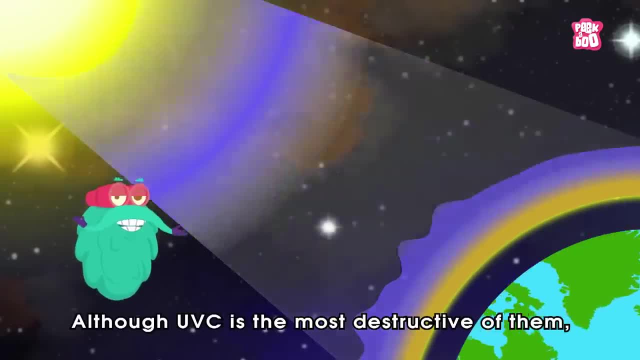 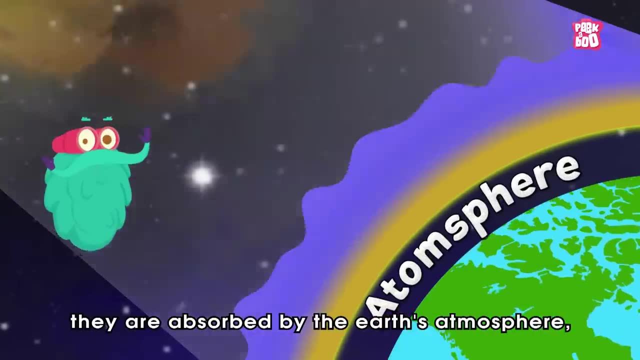 Although UVC is the most powerful ray. UVC is the most powerful ray. Although UVC is the most powerful ray, UVC is the most powerful ray And UVB is the most destructive of them. Fortunately, they are absorbed by the earth's atmosphere. 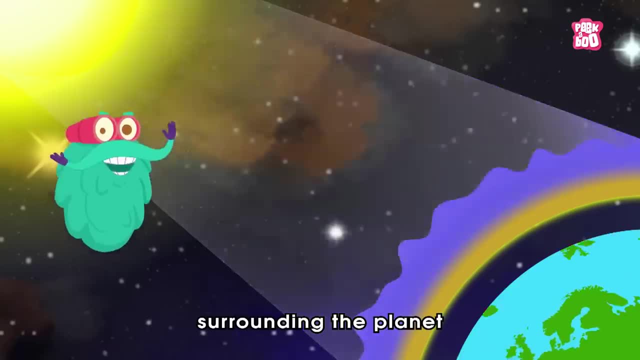 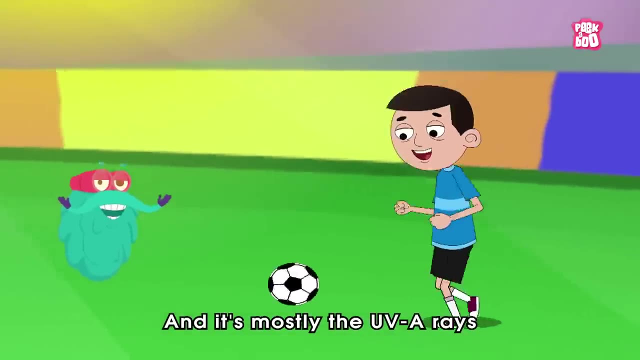 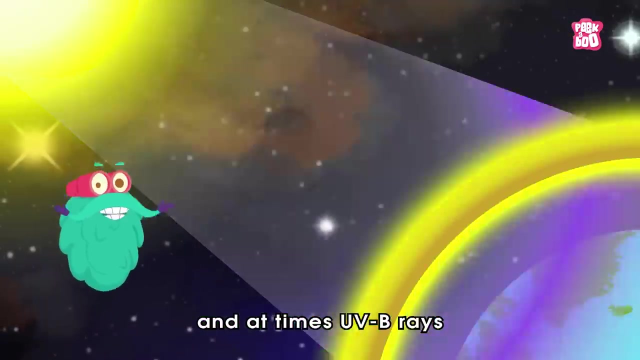 Which is the protective layer of gases surrounding the planet and does not reach the earth's surface, And it's mostly the UVA rays that we get exposed to on a daily basis, And at times, UVB rays can penetrate or come through the atmosphere. 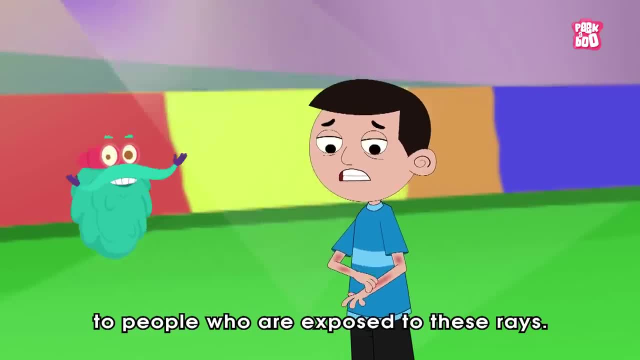 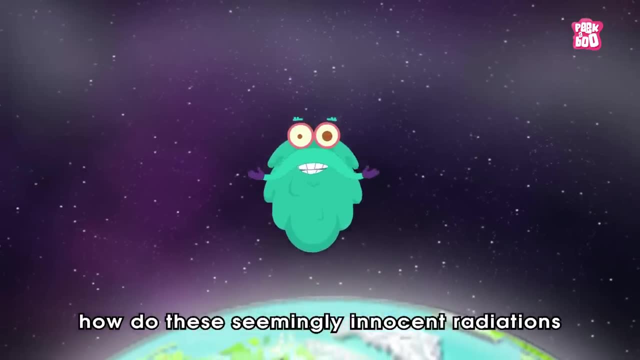 And at times, UVB rays can penetrate or come through the atmosphere. Those are the people who are exposed to these rays. Those are the people who are exposed to these rays, But the vital question is: How do these seemingly innocent radiations cause so much of damage to us? 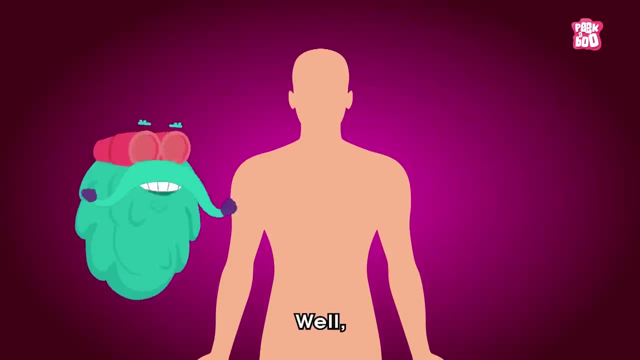 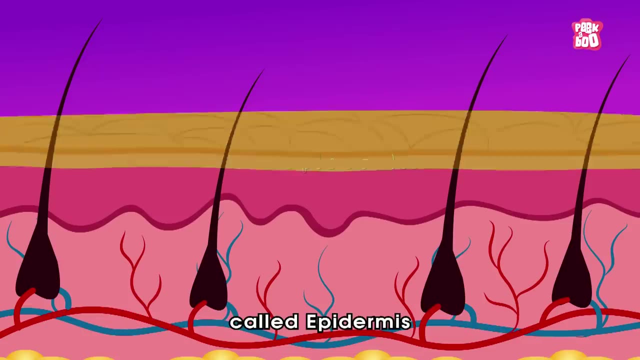 How do these seemingly innocent radiations cause so much of damage to us? Well, for that We need to zoom into your body To look at the upper layer of the skin called epidermis That protects you from many external forces, Just like that. 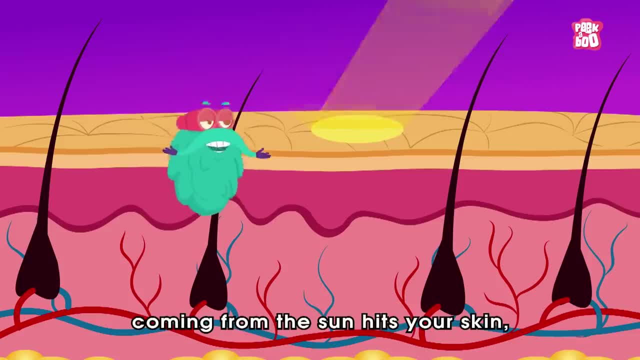 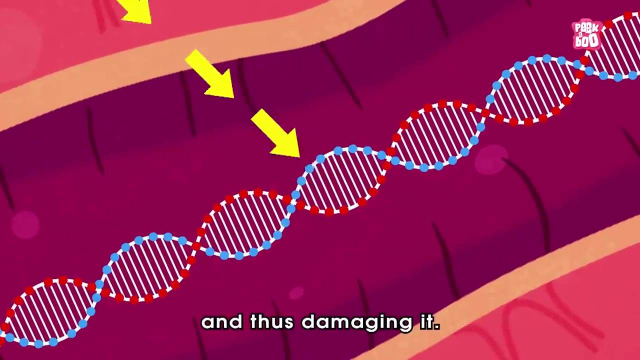 the UV light coming from everlasting seems to be having the effect of affecting your ideals, Just like that. When the sun hits your skin, it reflects off the epidermis, but the UVB can penetrate through your skin into the epidermis and reacts with the DNA and thus damaging it. 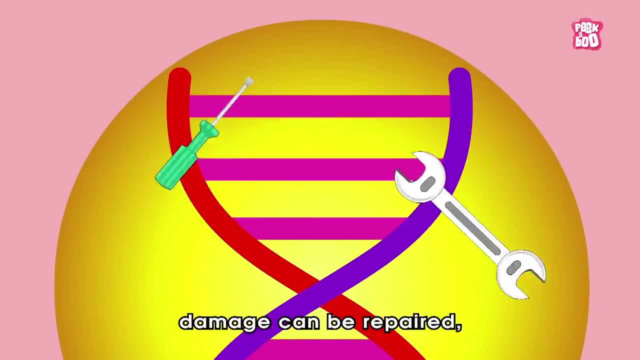 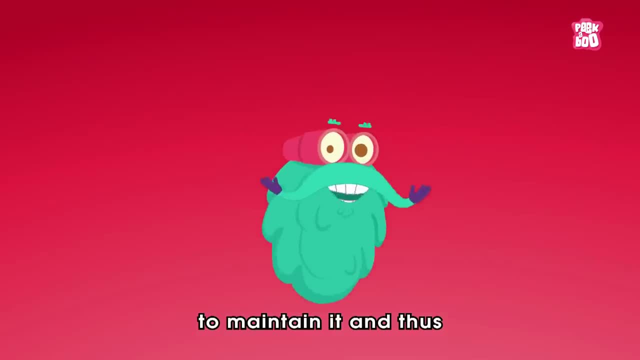 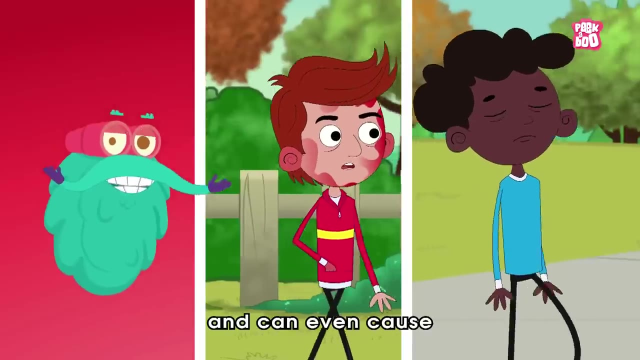 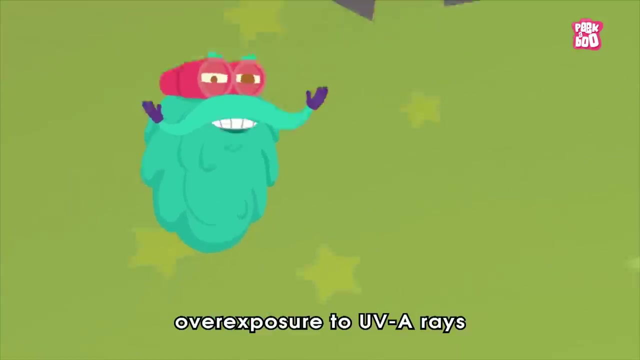 Although a low level damage can be repaired, but over exposure to UVB rays makes it hard for our body to maintain it and thus leading to many skin disorders, including skin burns, inflammation, and can even cause skin cancer. On the other hand, over exposure to UVA rays can also lead to cancer, but it is mostly 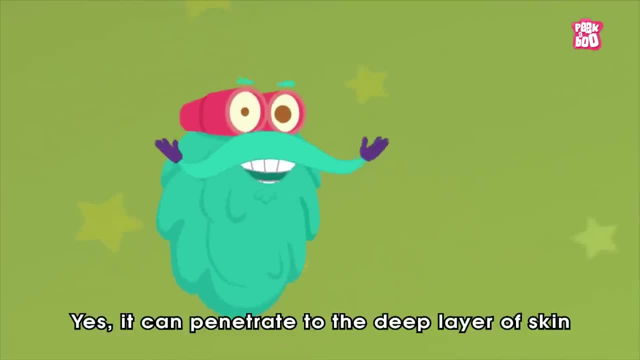 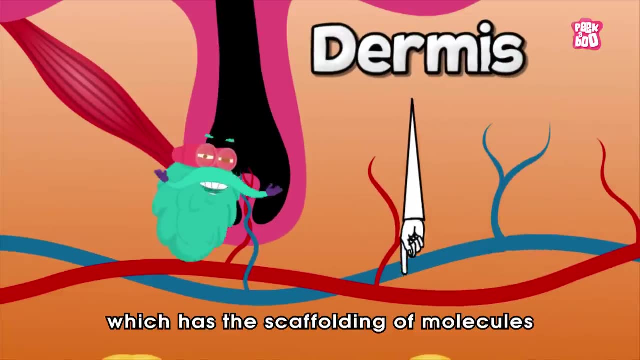 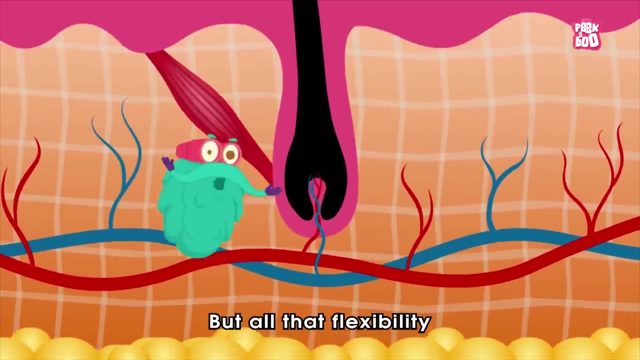 responsible for causing wrinkles. Yes, it can penetrate to the deep layer of skin. This is called the dermis, which has the scaffolding of molecules such as collagen. that gives your skin the elasticity, but all the flexibility finds it hard to fight the UVA rays as it 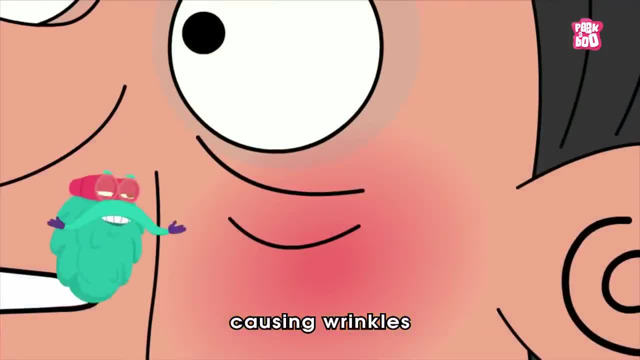 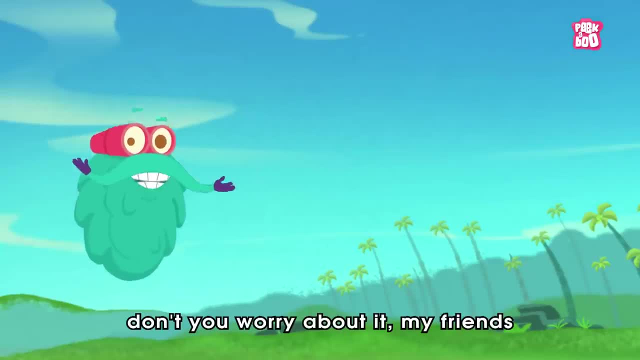 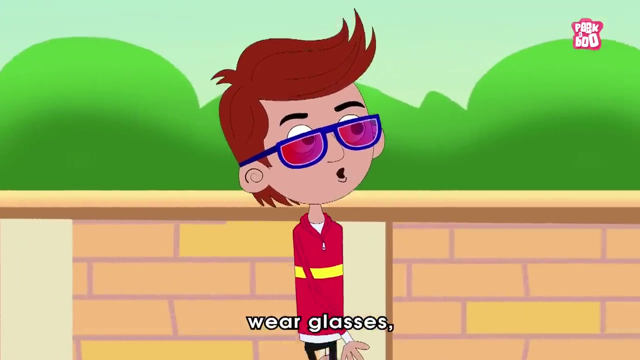 damages the collagen scaffolding, causing wrinkles and making you look older than your age. But don't you worry about it, my friends, As there are very easy pieces, Easy, lemon squeezy ways to protect ourselves from the wrath of the sun. Yes, just limit your time in the sun, wear glasses. 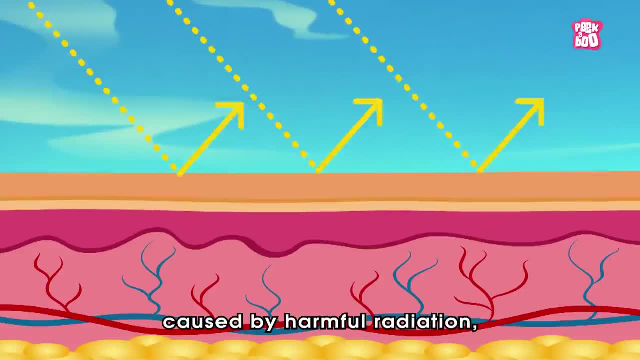 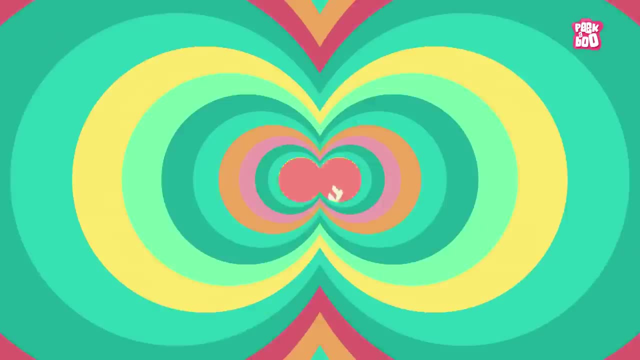 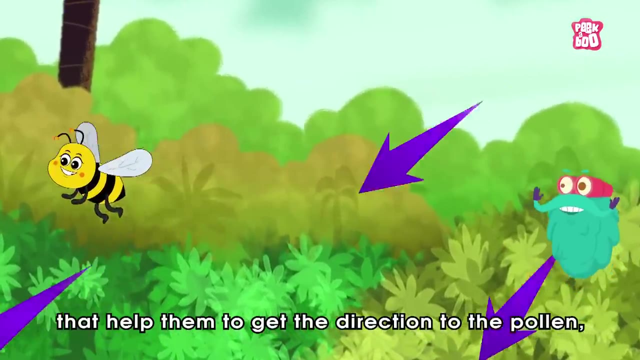 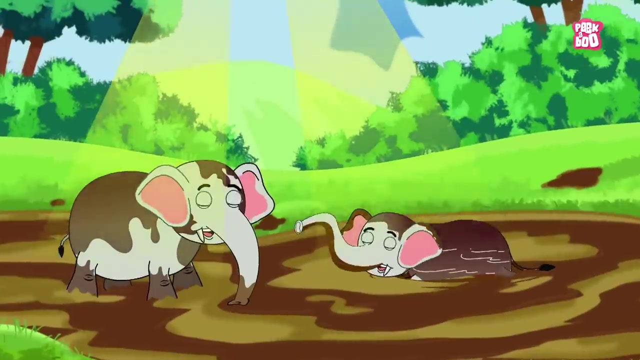 Using sunscreen can reduce the level of damage caused by harmful radiation and you can continue to live a healthy life. Did you know The bees can see the UV rays that help them to get the direction to the pole of their pollen, as the rays are reflected on the petals. 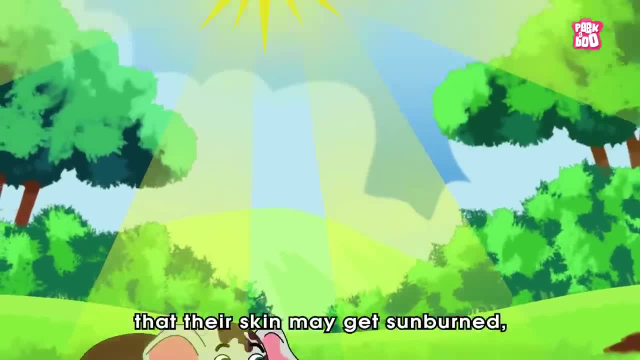 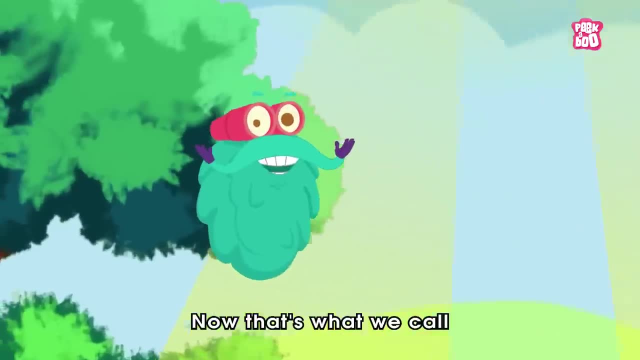 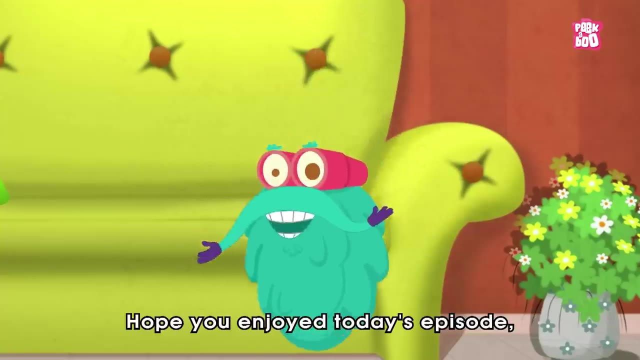 Also, elephants can sense that their skin may get sunburned, and hence they guard themselves by covering up in a protective coat of mud. Now, that's what we call being self-aware. Hope you enjoyed today's episode. Until next time, it's me, Dr Binox, Zooming Out. Ah, never mind.